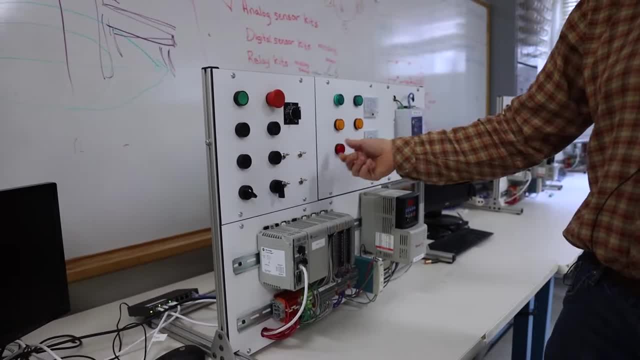 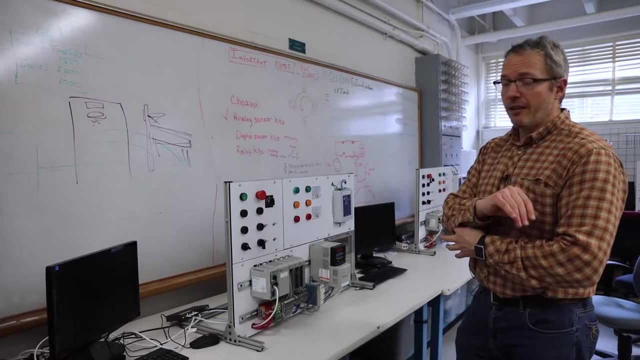 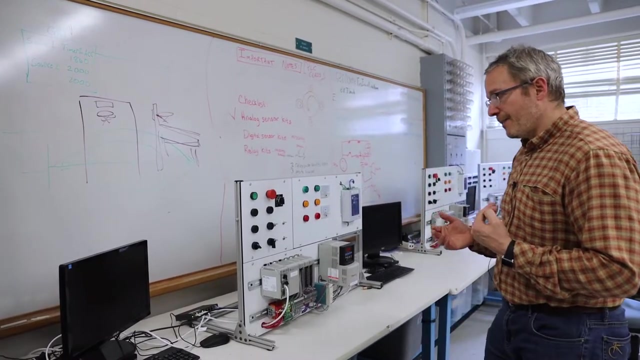 and then you verify that switches in certain conditions will turn lights on and off or turn meters and make things happen. So car companies use these because they allow a lot of flexibility for equipment And it makes it very efficient to make changes. Also, troubleshooting is really easy And you're 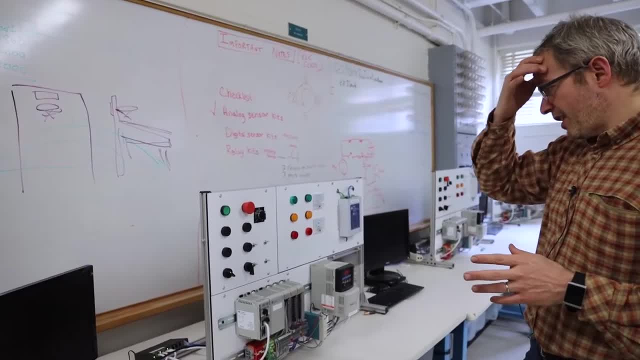 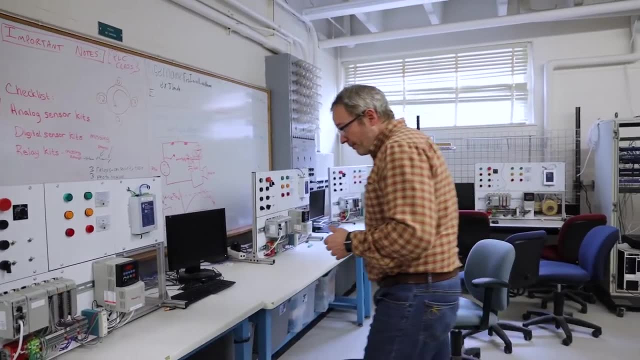 just gonna find that there's a lot of flexibility with this. So this is the industrial automation aspect of it, Using programmable logic controllers. we also have things where we can control the speeds of some motors And so, if you can see, in the back here we have a screen that you 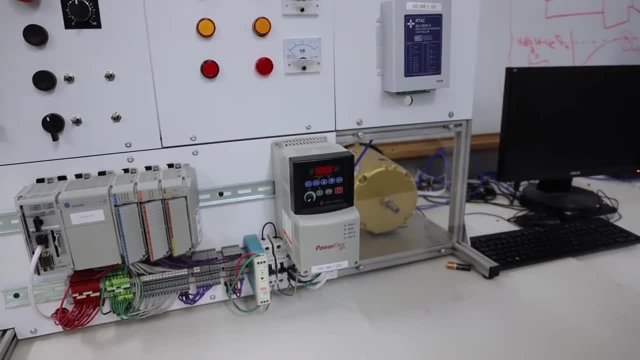 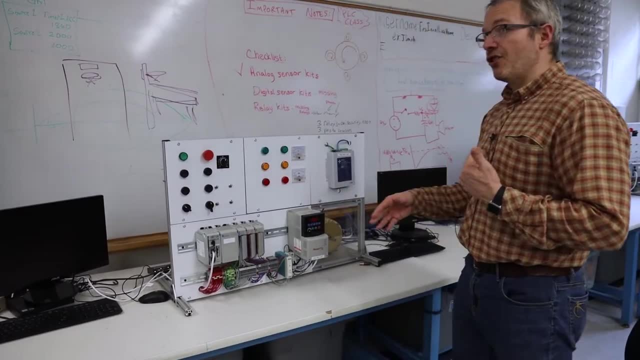 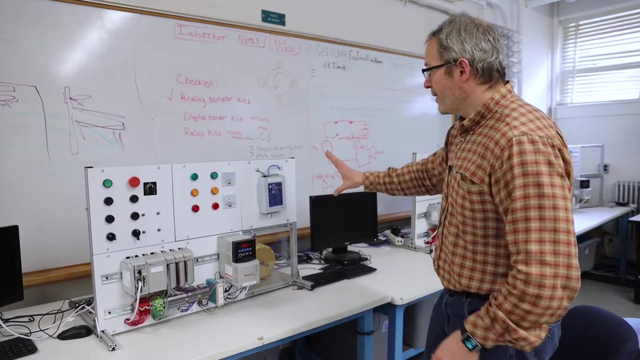 can protect your fingers, but we basically can adjust the speed of motors In an industrial facility. sometimes things are going too fast or too slow and this very frequency drive allows you to change the speed to enhance productivity, improve efficiency, utilize less energy, etc. etc. we also are pretty unique because we have these devices called 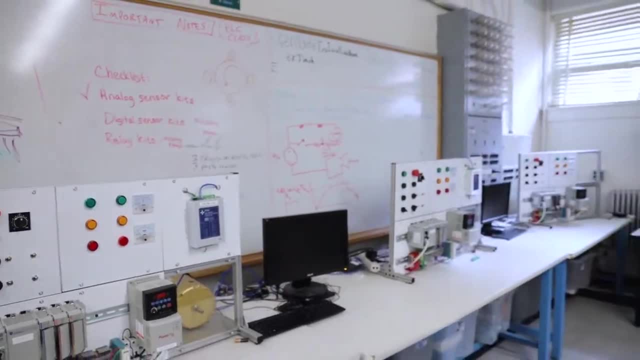 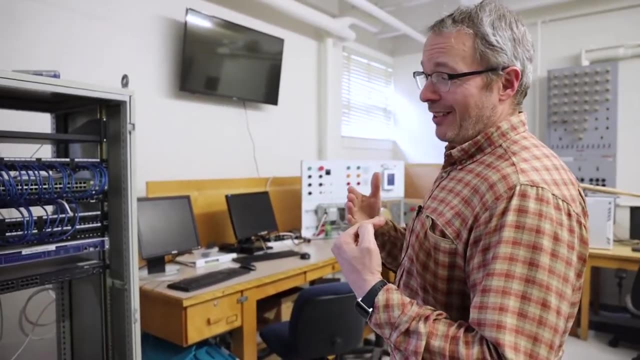 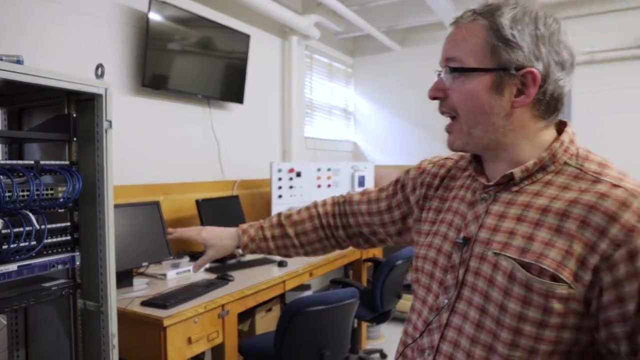 real-time automation controllers and those are intended to integrate into a server so that you can use an overall plant- what we call human machine interface, which allows us to really go ahead and get really nitty-gritty in managing an overall plant with individual devices. but at 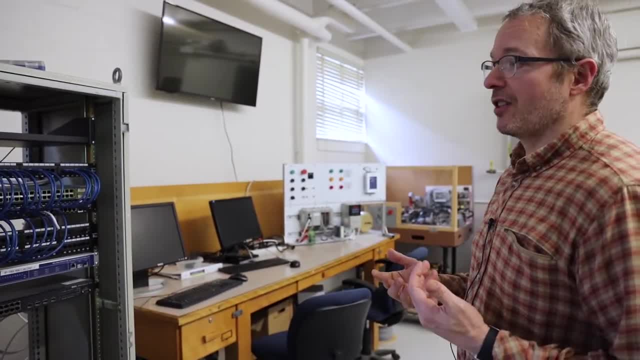 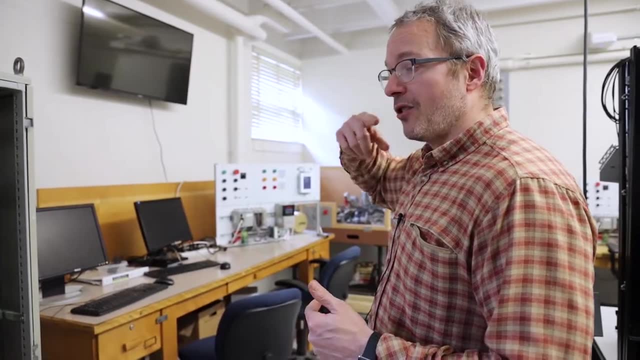 a higher level. so, for example, you could run an entire processing facility, a very large generating plant, with just a couple of operators in the control room and then have a few rolling operators just to make sure that there's not fires or things happening like that. so as we get more and more, 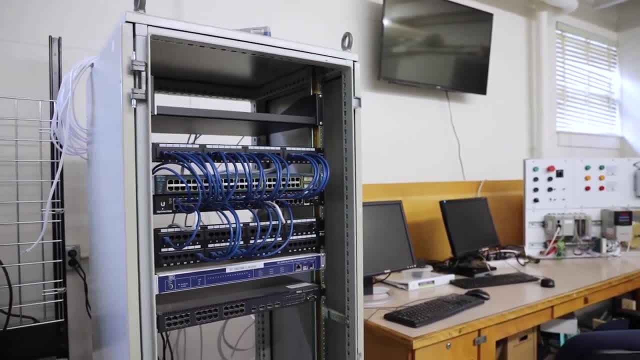 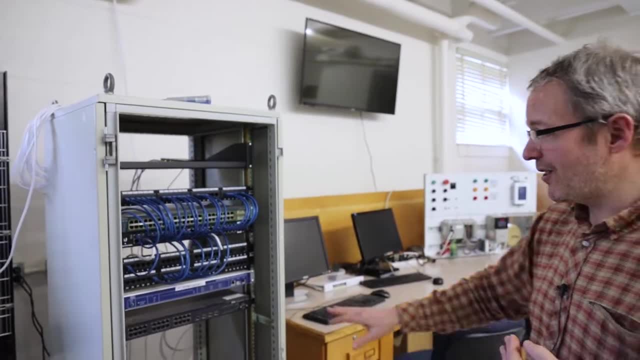 sophisticated with our automation, more error, more troubleshooting, more checking. it's going to make it so that we're more precise, we can get better responses and we can troubleshoot things much more effectively. so this is really a unique part of our program and not a lot of programs across the 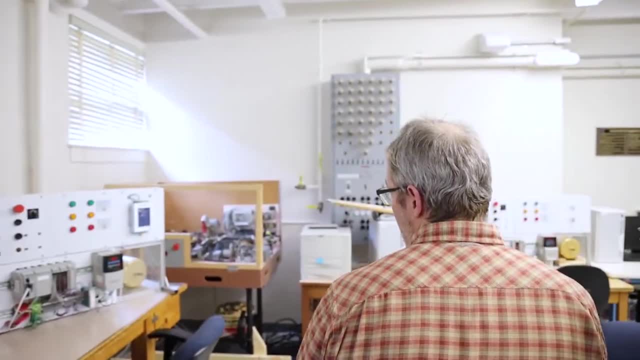 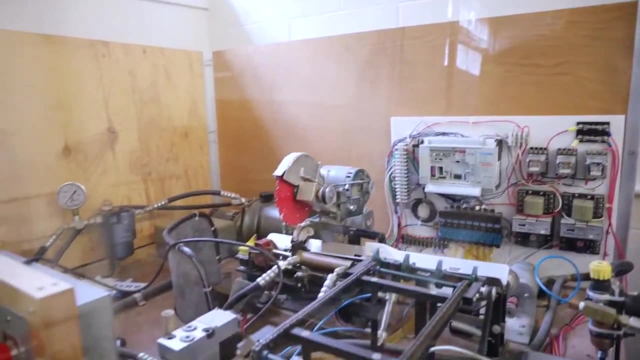 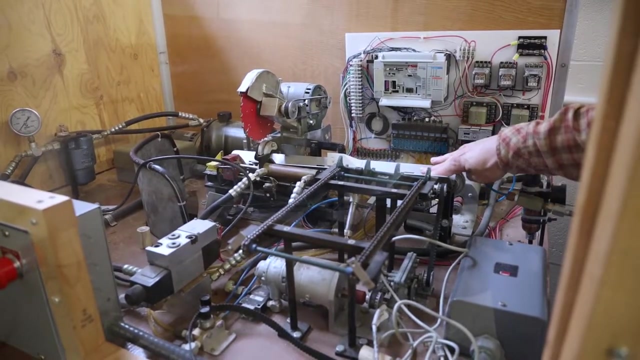 country have this capability. um, you can see here kind of a scale model of an industrial facility. this is essentially a facility that converts wood products into firewood. so you have scale logs which would be dowels that would be on this assembly. they ride through here and you can notice a sensor. 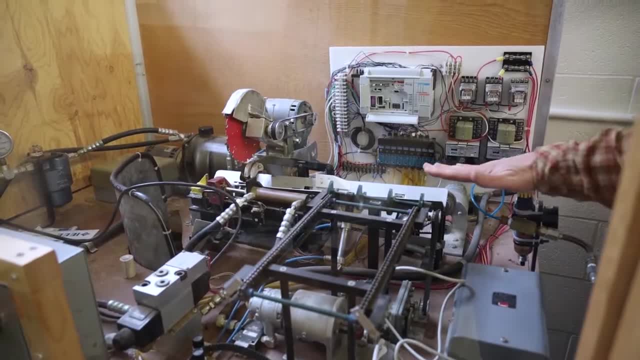 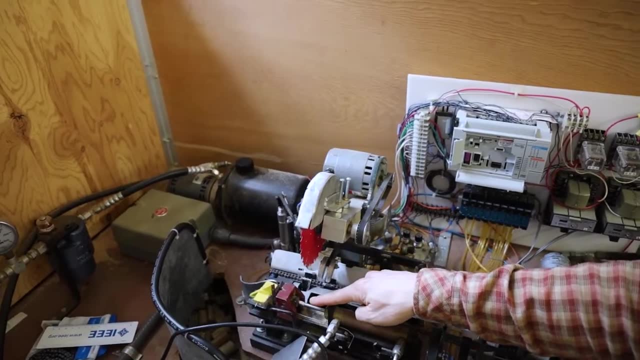 here to detect that there's an actual log, and then that log will traverse through. it'll be held in position and the saw comes down and cuts it to length. it gets ejected into this spot where you have this hydraulic ram, and then the saw comes down and cuts it to length. it gets ejected into. 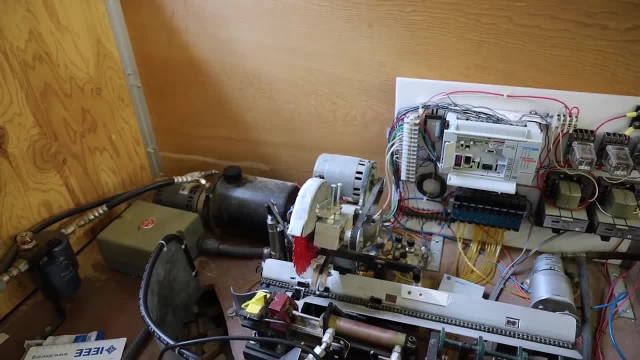 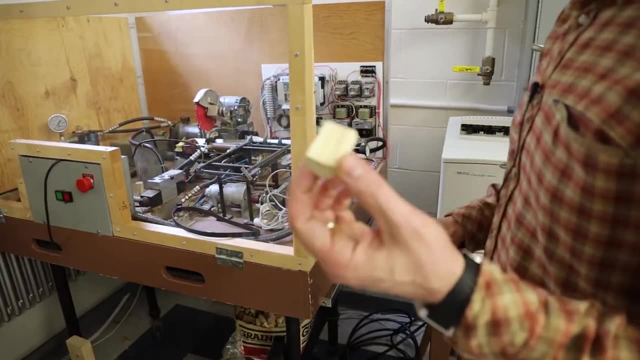 this spot where you have this hydraulic ram that drives it and then pushes it through the splitter and then hopefully you get fairly well cut and split pieces of wood. so this is a dowel that's been cut in half but get you get the sense of it, and so this is really interesting because 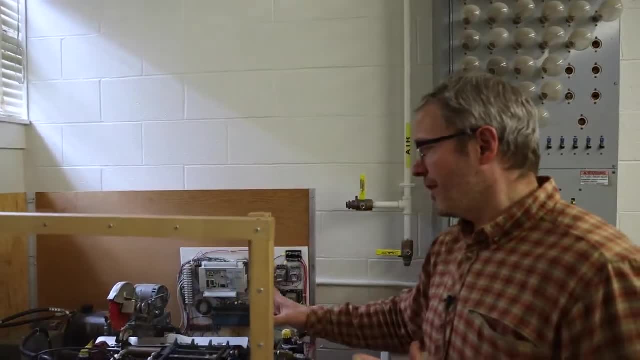 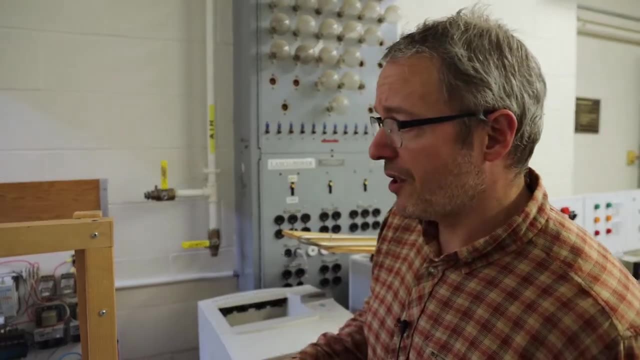 it allows you to build systems that are mechanical. you can see, this is a really big mechanical process, but all the brains and all the control are done with electronics and as we get more and more sophisticated with our controls, more and more work is going to be done. 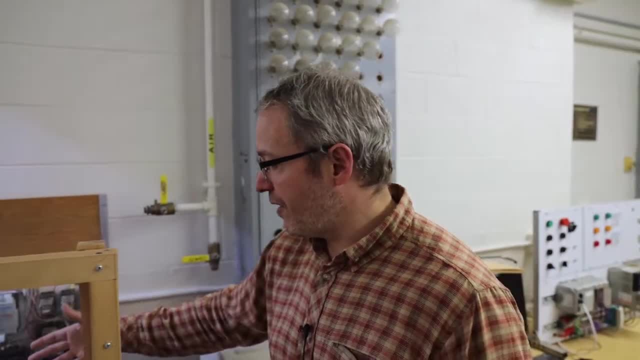 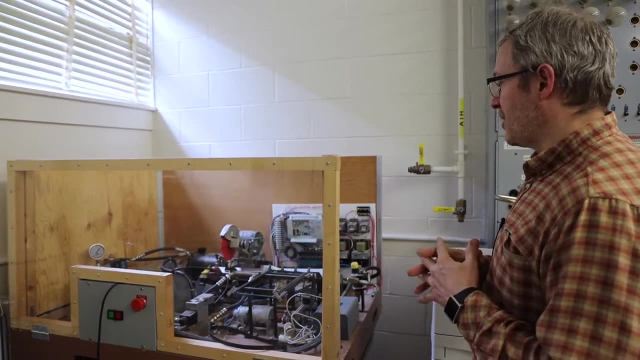 with electronic controls and whatnot. so this is a fair amount of hydraulics. you're starting to see more and more of this is being done with electric circuits as we get more power, better efficiency, more improvements and, yeah, we're getting a lot of improvements, a lot of. 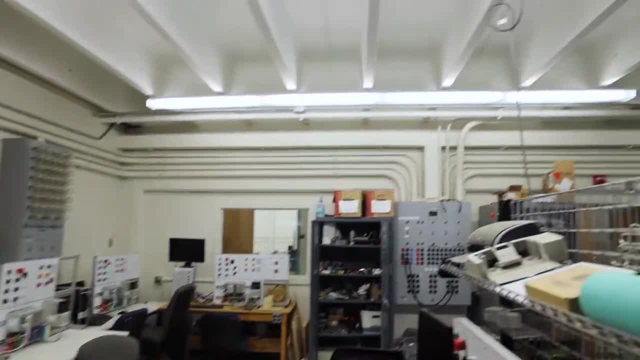 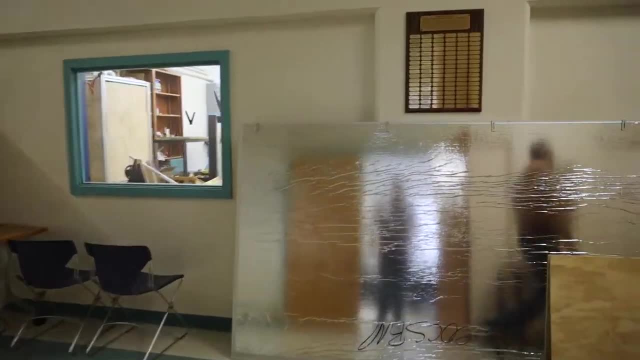 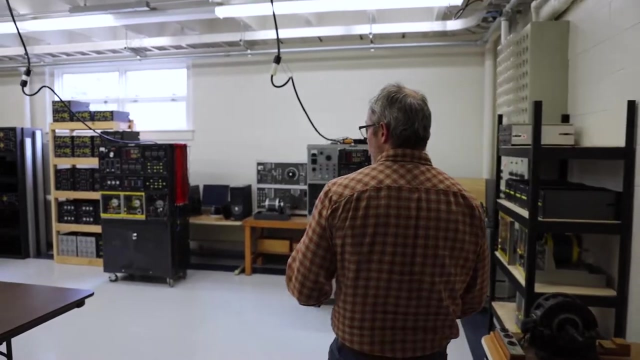 changes. let's move on to our next lab, which is the lab that we get to demonstrate some ac circuits and we get to build. we get to build some circuits that are going to be real world. so, the utility power system, what's coming into your house? it's what's. 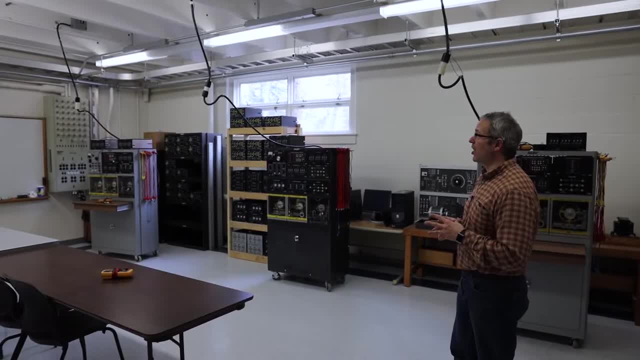 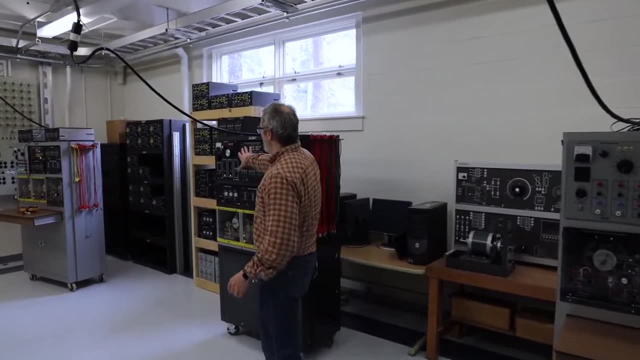 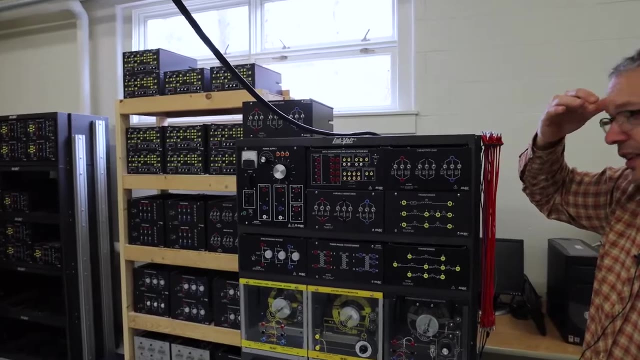 called alternating current and in this lab it's pretty much focused on alternating current systems. so we have six stations and each of these stations are more or less configured the same. we have a variable three phase power supply. we also have some dc, because some of the equipment that we have here actually need a dc field to be able to drive things. 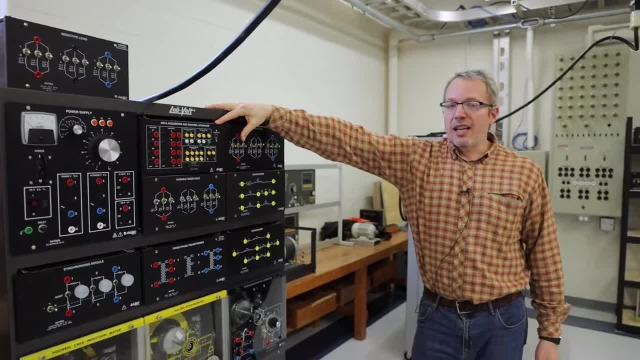 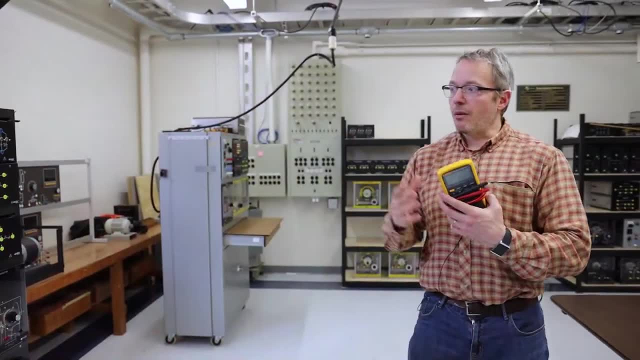 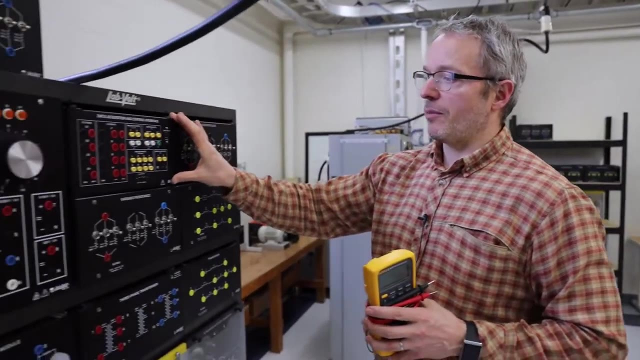 we also have a pretty fancy metering package, which is this data acquisition, which converts your into a very, very, very fancy multimeter. so what that allows us to do is do way more sophisticated analysis and understanding of the circuits by using your computer to look at waveforms. so 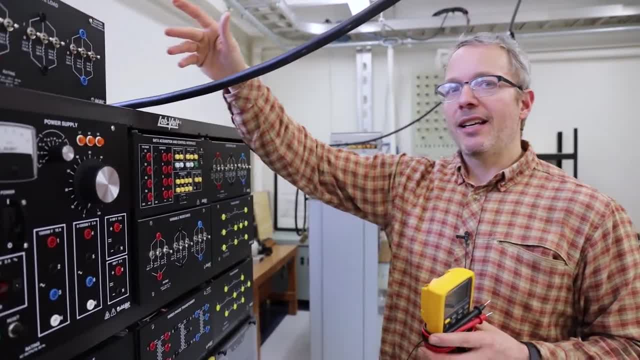 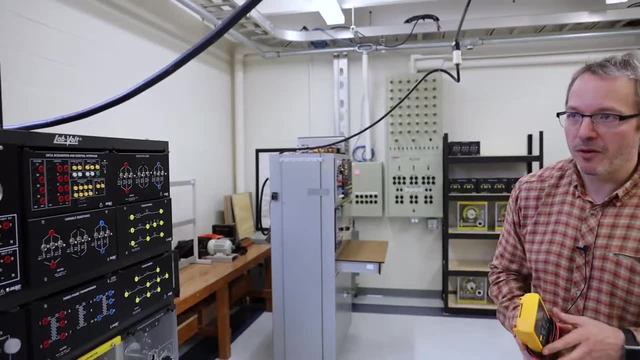 these modules. you can swap them in and out pretty easily and it just allows us greater flexibility to try different tests of equipment. so if you were to look around the perimeter of the room, you'll see all kinds of different modules and how we can change these things out. so this is a 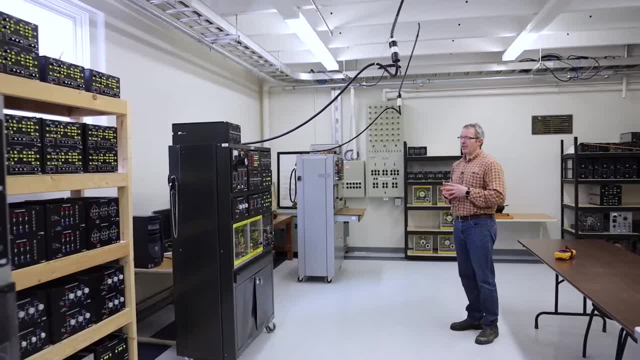 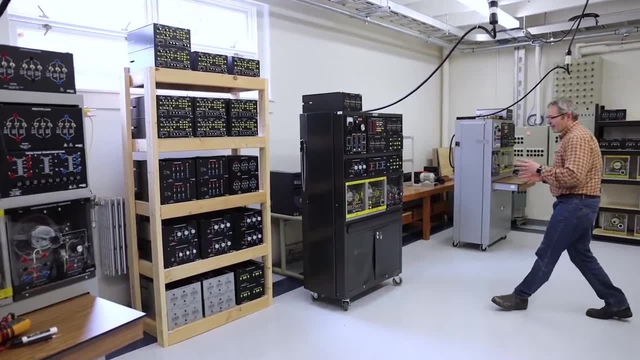 lab that you'd be using perhaps in your sophomore or even junior years, and also some of our students and senior projects will use some of the equipment in this lab to go ahead and test it. nice thing is it's very safe. we have good guards here. all of our wires have guards associated with them. 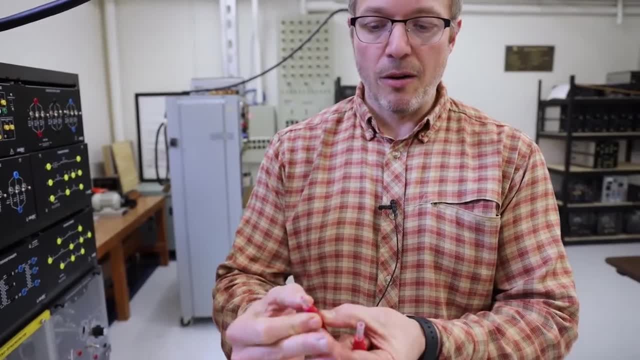 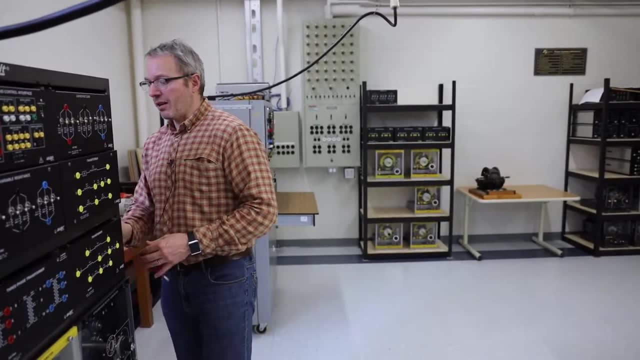 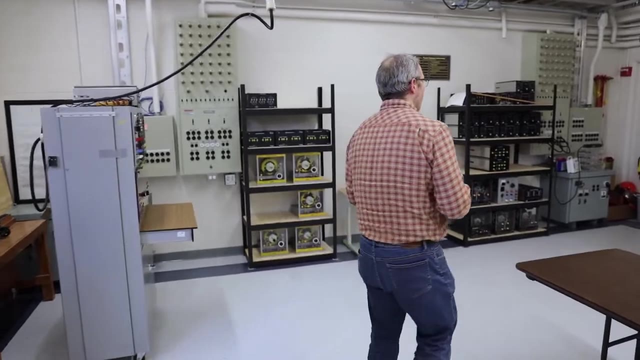 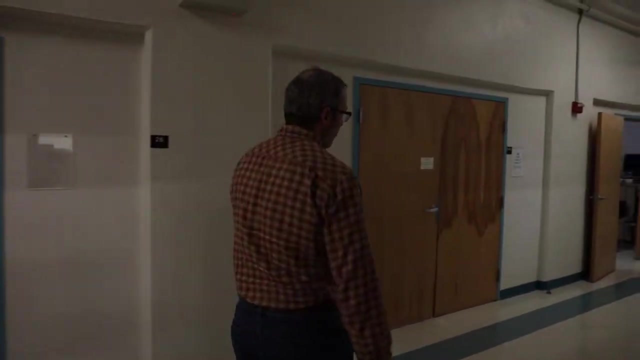 you can see that we have nice shielding so you are prevented from coming into contact with any of the live parts. so really nice lab so we can work with real power, but we don't have to expose ourselves to anything dangerous. so a very safe environment. let's go look at our senior project lab. and this lab is intended to be a mess. 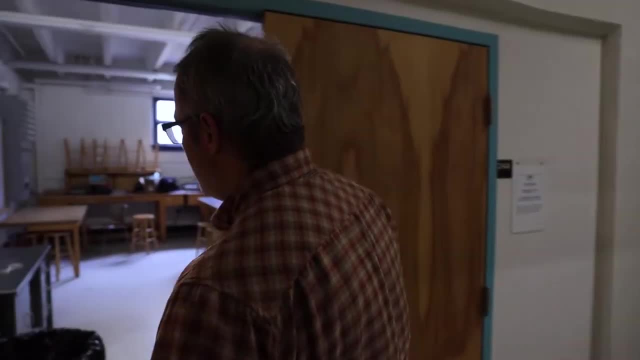 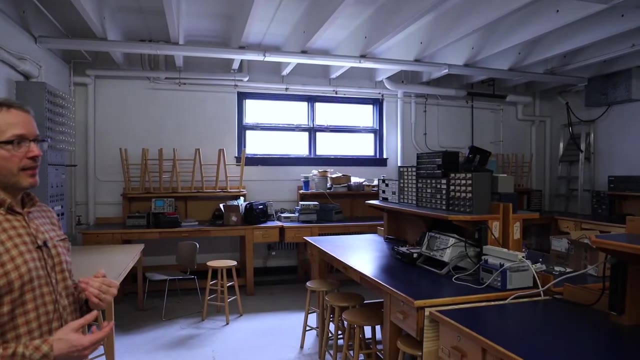 because this is really a student-run lab where they build lots and lots of projects. you're going to spend three semesters in here designing something that demonstrates what you've learned through the program. it's called a capstone experience, so as a capstone experience you get to. 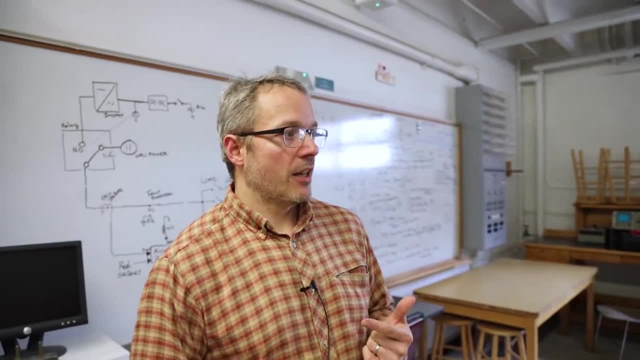 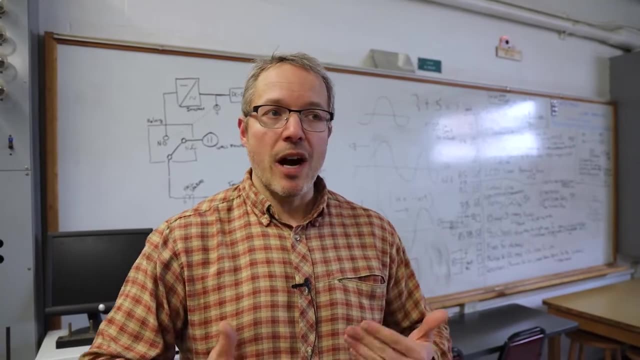 what would i like to build? so you pick a project and then you demonstrate that it meets your specifications, and then you get to demonstrate it to your class so it really gives you, you know, sort of that sense of accomplishment. wow, look what i've learned in the four years that i've been here. i've 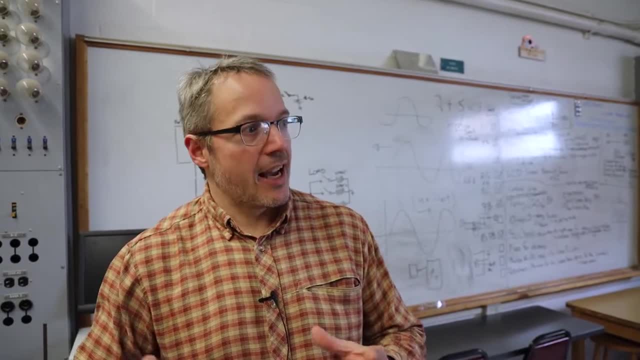 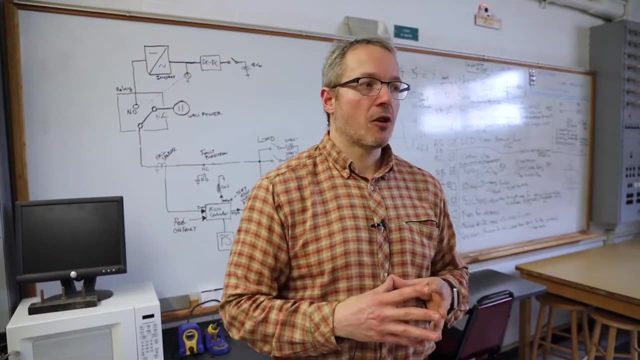 been able to take. you know what little math and physics understanding i had, and now i can build this really cool circuit that can control the speed of a motor, or can monitor a parking lot and determine where parking spots are available, or, you know, can enhance capture of photovoltaic energy. 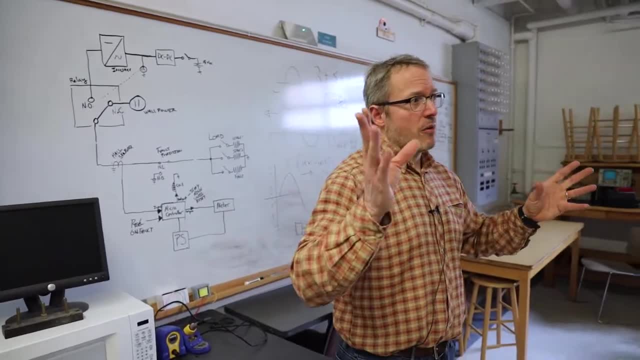 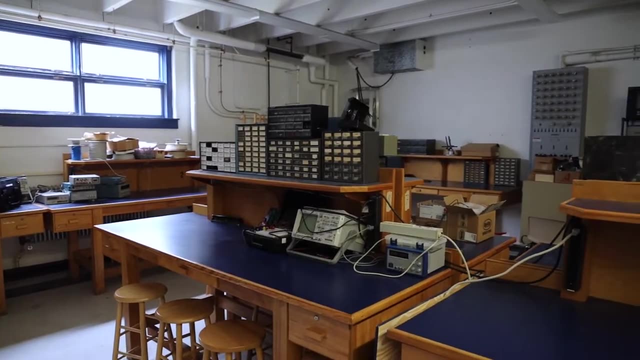 so lots of components here, all kinds of equipment, everything is sort of spread out, but again it's. it's not meant to be a junk room per se, but it's meant to have a lot of equipment, and if you need something you just grab it out of the cabinet and see what works. and so this would be your junior. 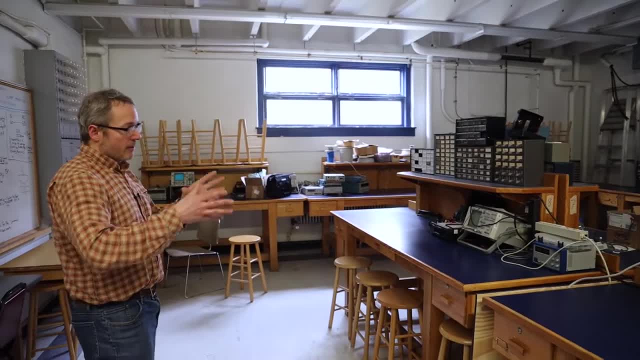 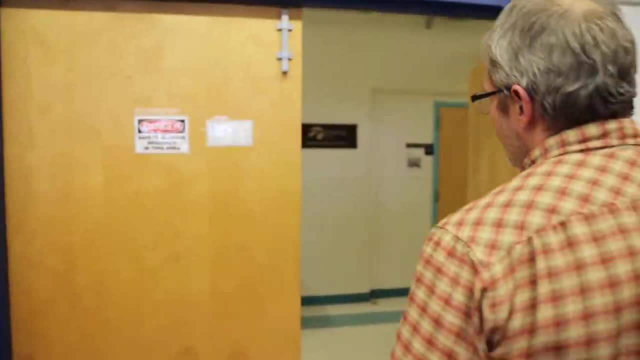 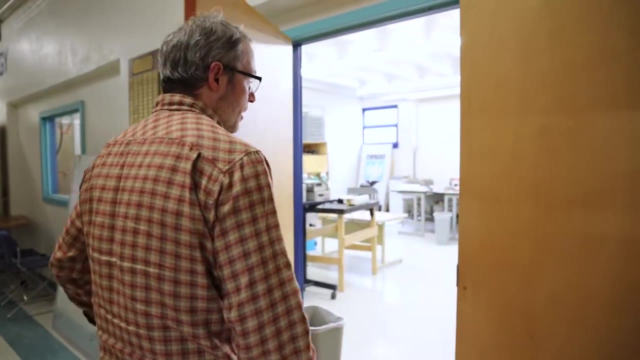 and senior years, where you get to go in and grab a bench and it becomes your space for that period of time. let's go into the next lab, which has another really unique project part of the program. so i'm a utility person by experience and our graduates really get picked. 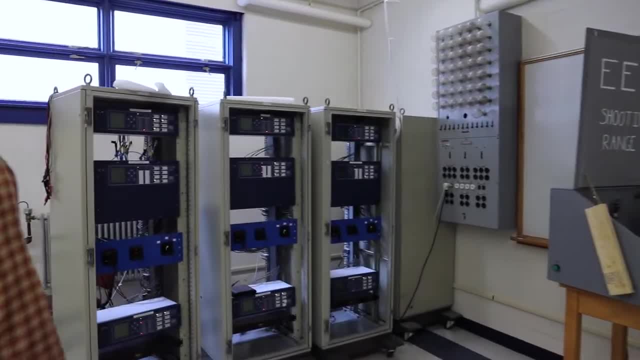 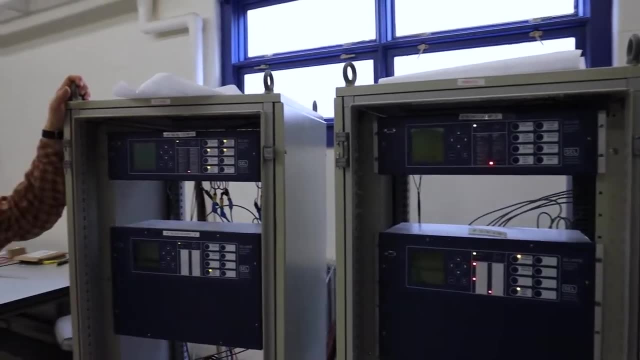 up by the utility world and it's mainly because we expose them to real world, practical devices. so if you were to go to any utility substation or any process area that has power generation utility, you would see lots of these devices. these just happen to be schweitzer engineering. 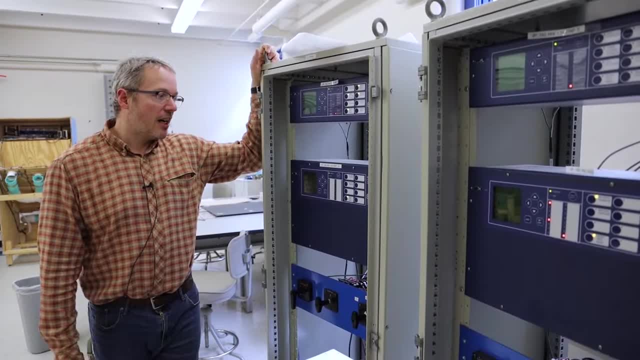 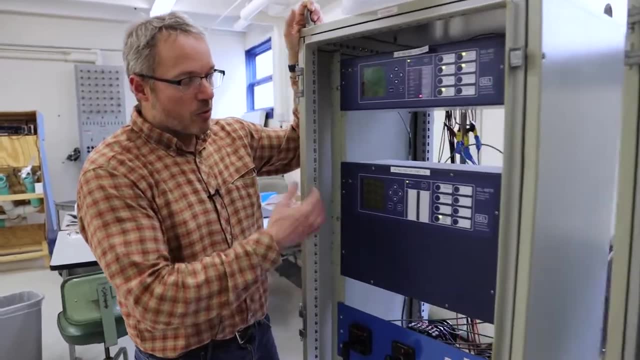 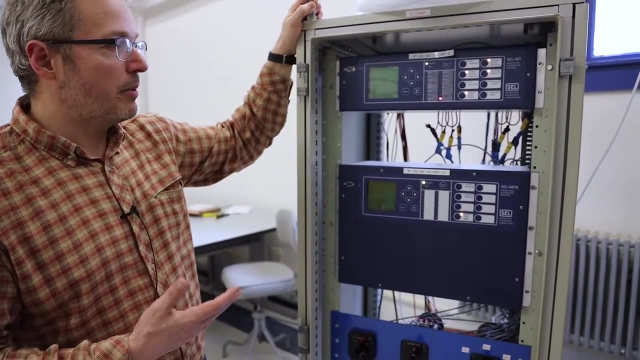 laboratories equipment, but a lot of the philosophies apply to uh any manufacturer, general electric, abb, etc. etc. so this is: if you have a real world utility system, they monitor the same exact parameters we do and they will issue trips to protect the line, maintain high reliability but remove faults from out from service. so we have these and there are. 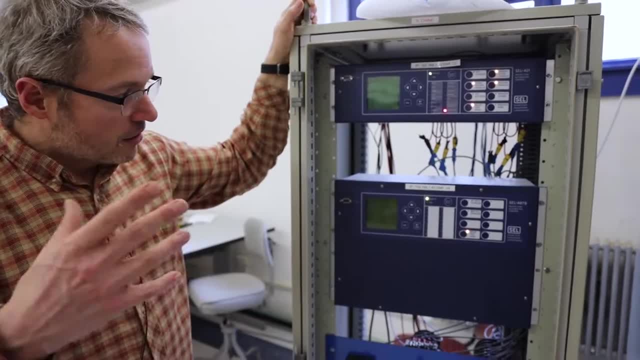 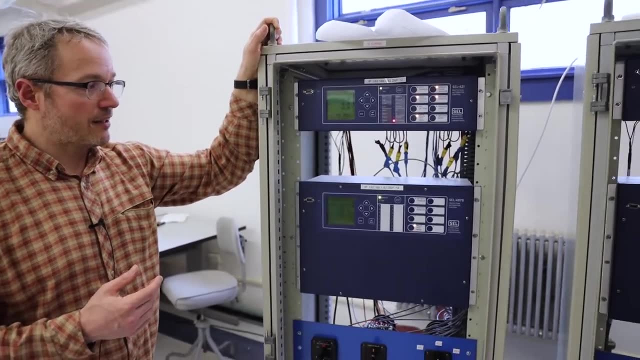 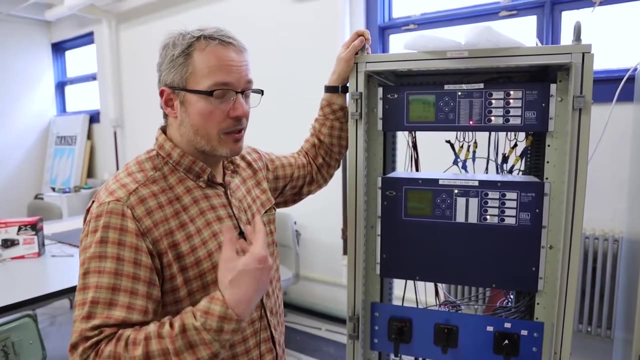 three identical stations so you get to actually put your settings, check that they work, make sure that everything goes as intended, and you get to get real familiar with these particular devices, so very unique. we have these. a lot of institutions are trying to get more adapted into relaying but because we've 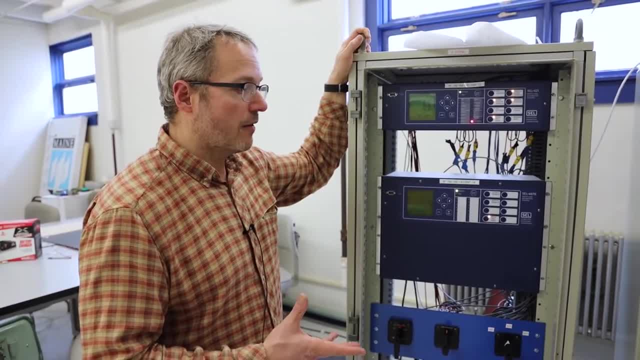 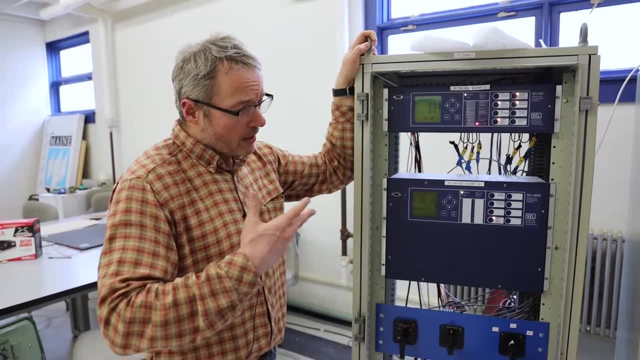 got these boxes and we get a lot of industry support. we do very, very well with explain these topics and this is a really in demand part of our, of our program, and we've had a number of people that hire our students say you need to have them take all, everybody take this class, because they've 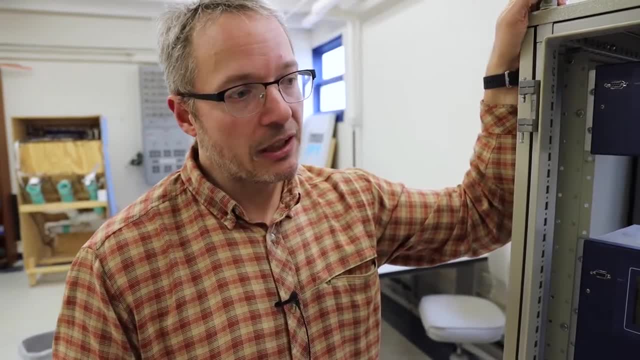 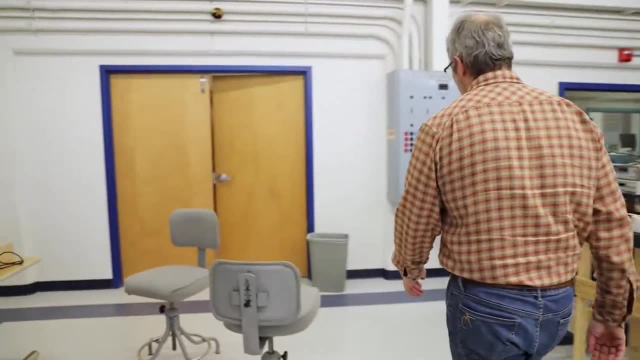 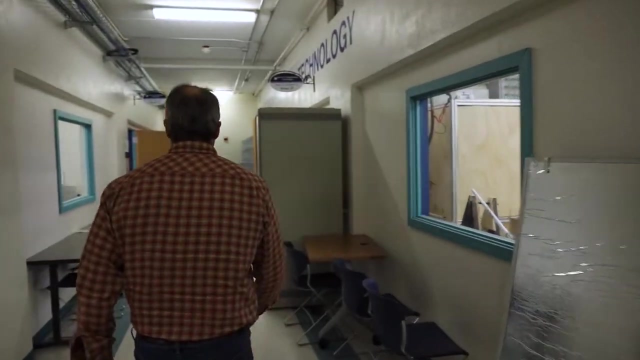 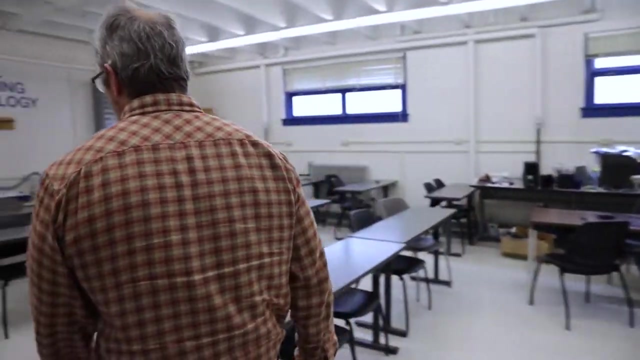 got such a great set of skills that they pick up by doing this relay lab part, so very, very powerful part of the lab. let's move on to the printed circuit board lab. so this is a smaller part of the program but it does a very effective job of showing you how your cell phone 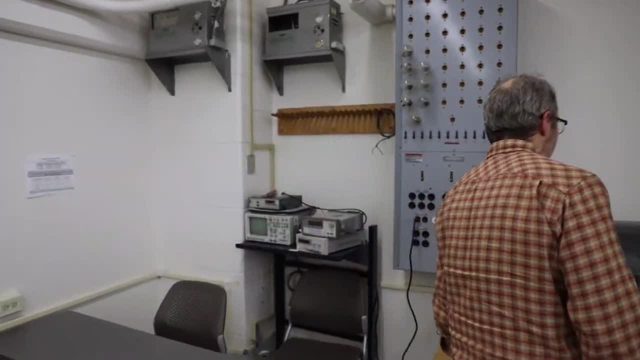 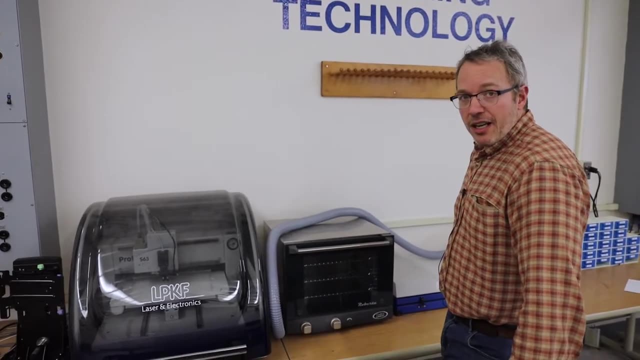 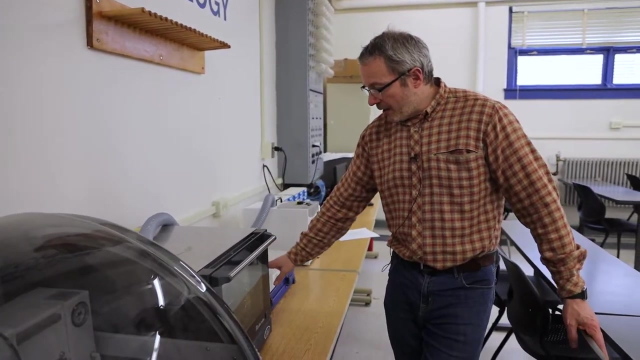 pretty much any handheld device how you can minimize the size and the energy consumption by doing what's called a printed circuit board, and so essentially, you can design a printed circuit board. we have a class that you design a printed circuit board and then you can use a uv device that actually will. 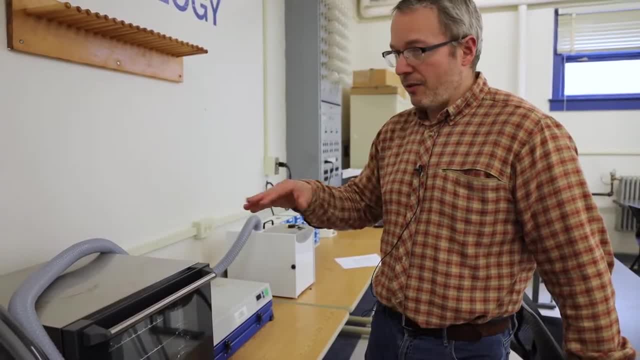 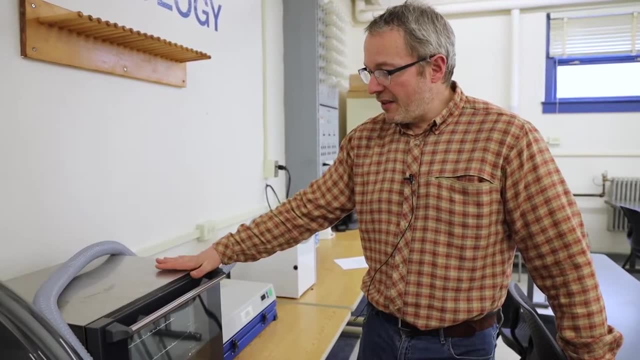 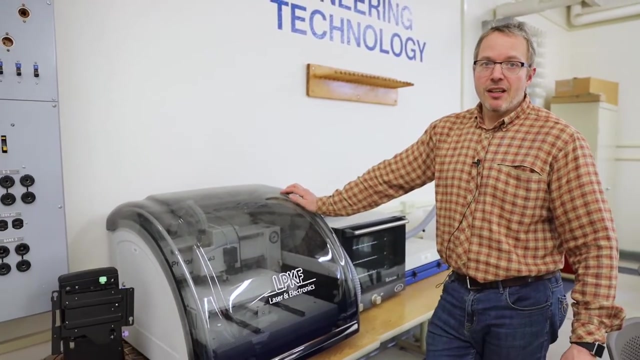 put your layout of your circuit board onto, essentially, a copper bus or copper plate, and then you bake that in the oven so that it stays in place, and then you use this milling machine to go ahead and remove any of the copper pieces that don't want to be there because you don't want to. 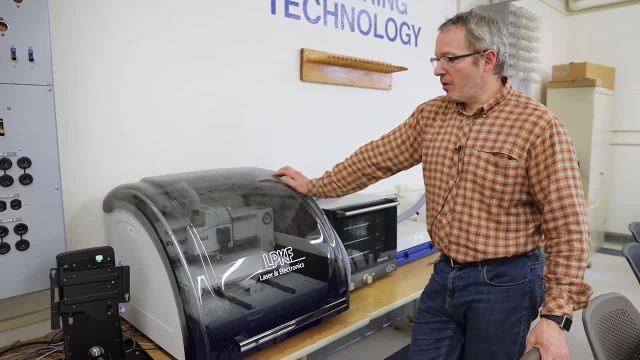 have connections between devices that are not connected to the circuit board. so that's a really useful piece of equipment and it can be used to do a lot of work to find connections between devices that don't belong because the circuit won't work as intended. so again another really nice distinctive.